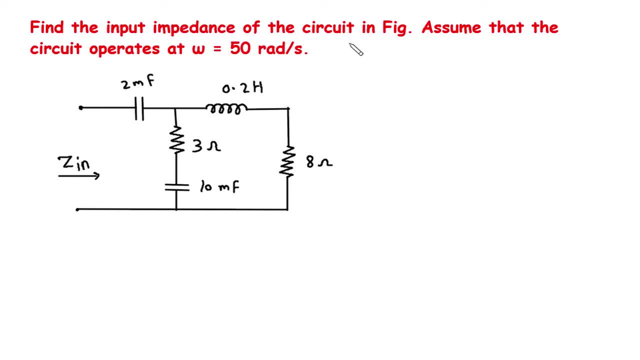 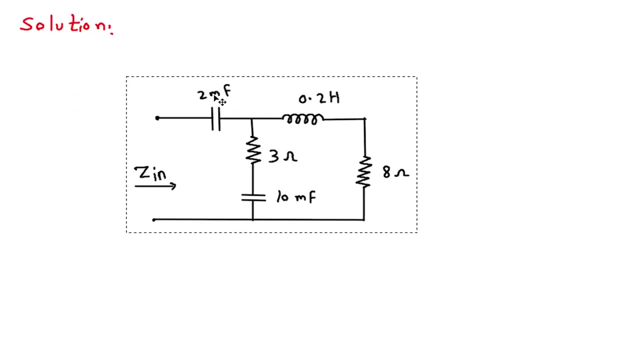 Find the input impedance of the circuit in figure. Assume that the circuit operates at omega is equal to 50 radian per second. We have to find this input impedance Solution first. we will redraw the circuit Now. let's say this is Z1, impedance Z1 and. 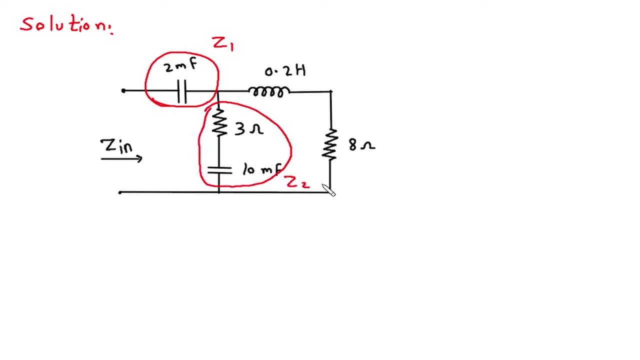 this is impedance Z2 and this is impedance Z3.. This is Z3.. So from this we can say Z1 is equal to 0.. This capacitor, only this, will be minus jxc. This is xc is the capacitive reactance. So 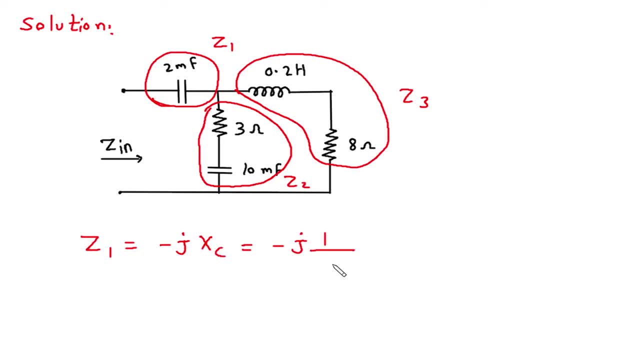 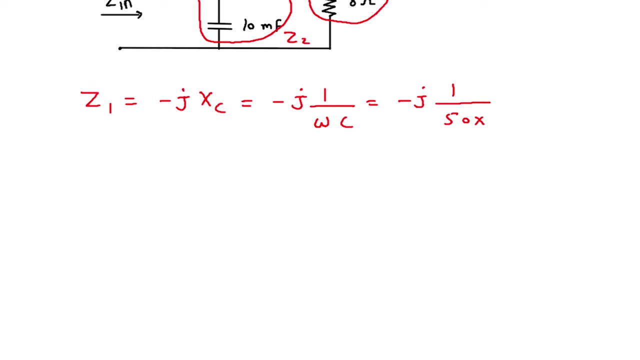 minus j. formula for this xc is 1 upon omega c, So this will be minus j into 1 upon omega. Omega is given that is 50 radian per second, So this will be 50 into. capacitance is 2. 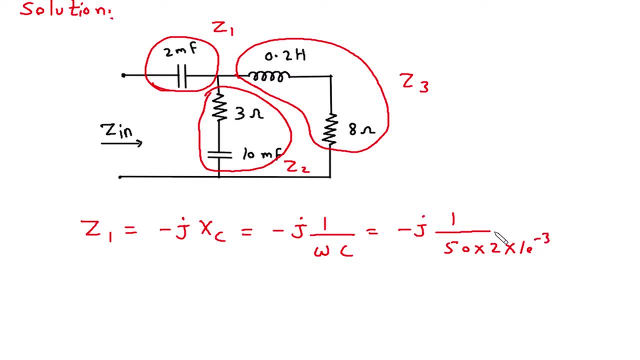 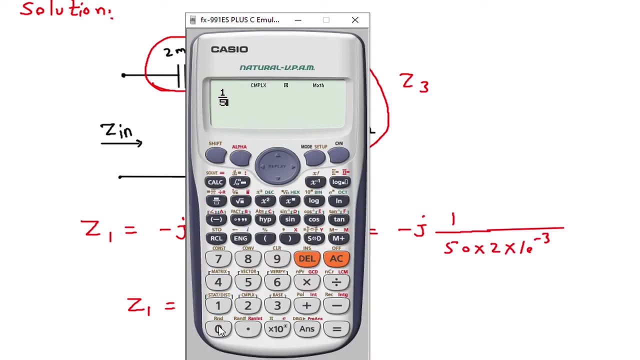 milli farad. So this will be 2 into 10.. the power minus 3.. So from this we can say z1 is equal to minus j, and this will be one upon 1, upon 50, into 2, into 10, to the power minus 3.. So it is 10.. This is the value for. 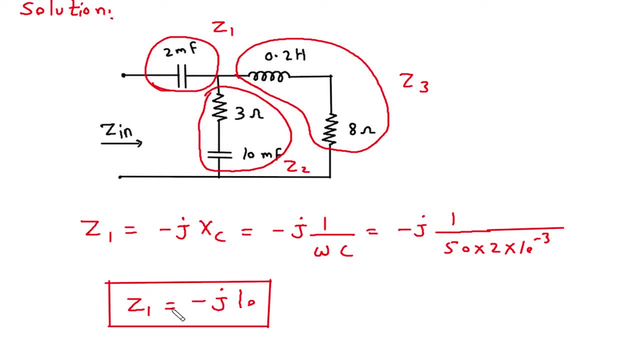 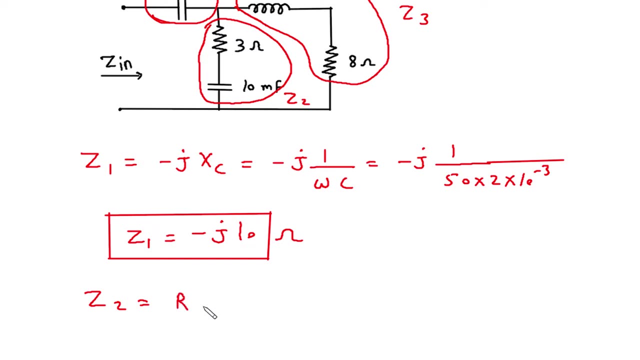 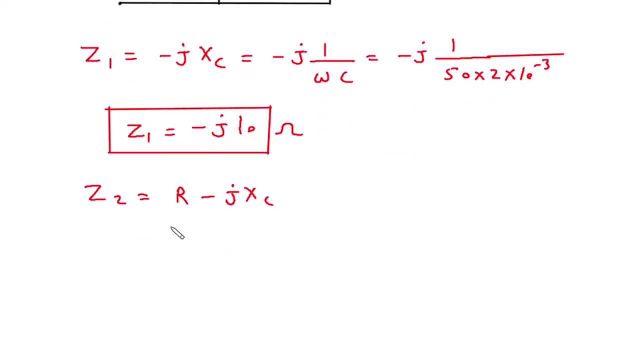 z1.. Also the unit of impedance is ohm. Then this Z2. here Z2 is in series with resistor and capacitor. Z2 is the series connection of resistor and capacitor. So we can write R plus, R minus, J, X, c. So this will be: resistance is 3 ohm and resistance is 2 ohm. 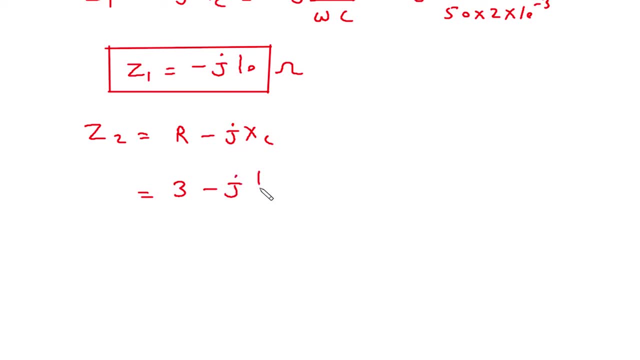 So J, 1 plus R minus J. X c is in series with resistor and capacitor. that was Z2.. So z2 is Theta able to vamp up resistor and capacitor and capacitor. that is one upon 50, and then So 3 as it is minus j. as it is again, formula for Xc is 1 upon Omega C. So this will be. 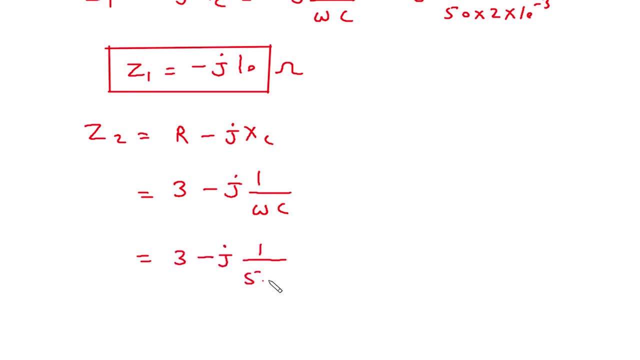 3 minus j 1 upon Omega is 50 into capacitance. Capacitance is 10 millifarad, so 10 into 10 to the power minus 3.. This will be 3 minus j 1 upon 50 into 10 into 10 to the power minus 3.. 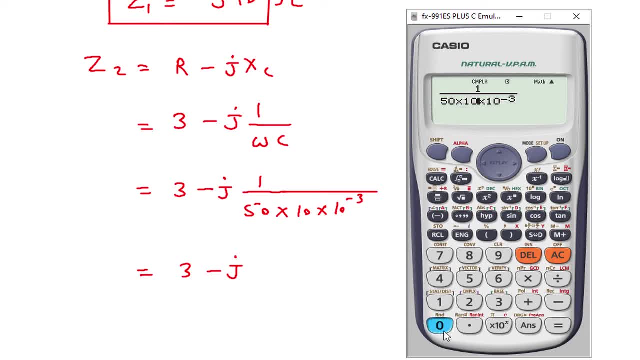 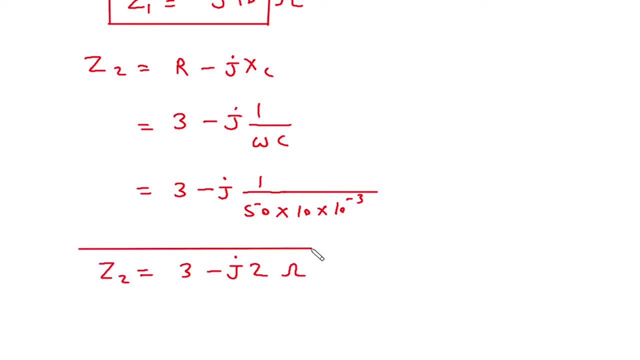 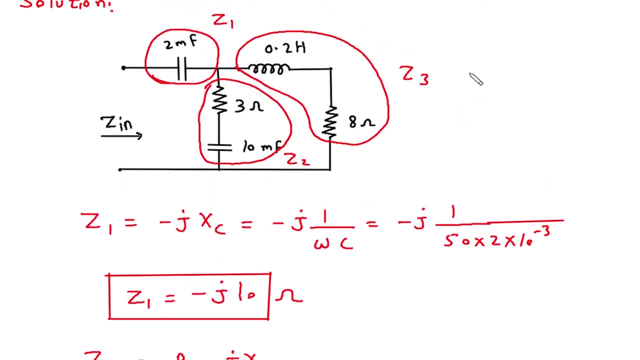 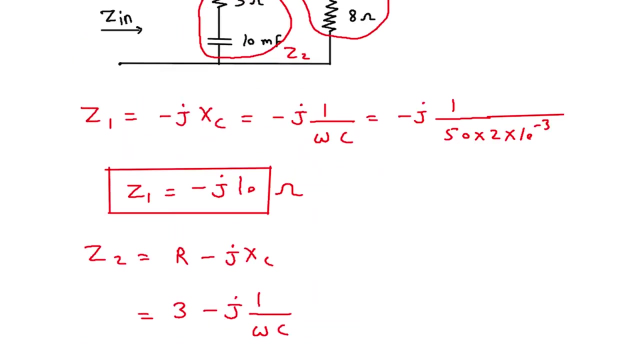 So here this will be minus 10 now, so it is 2.. Again, the unit is ohm. This is the value for Z2.. Next, Z3, this Z3 is equal to. here we will write: Z3 is equal to resistance plus inductance. 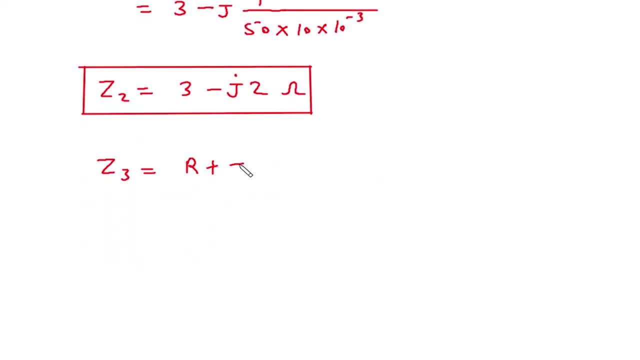 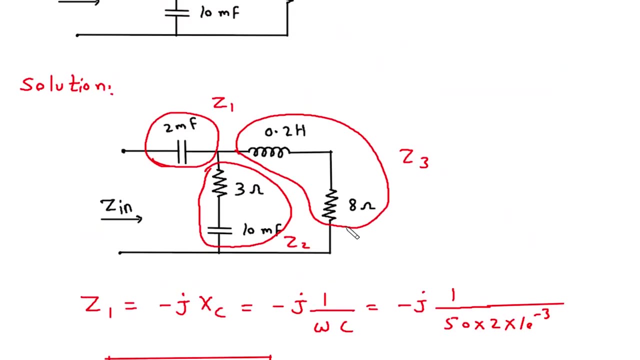 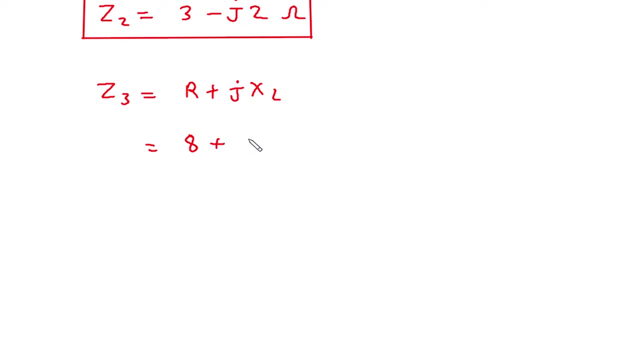 So R plus R plus j, xl So R. the value for R is 8 ohm and inductance is 0.2 henry. So this is 8 ohm and j as it is formula for this, xl is Omega, l, l is 0.2. 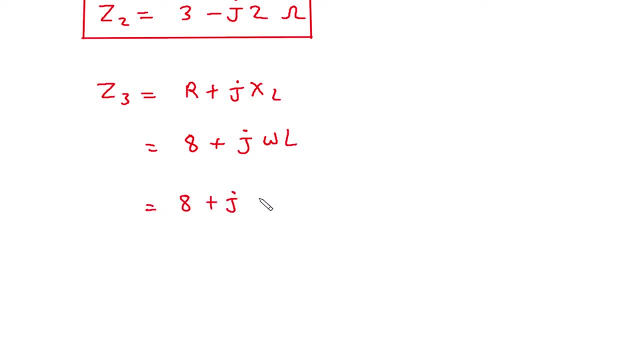 So this will be 8 plus j. Omega is 50 into 0.2.. So this will be 8 plus j. this 50 into 0.2 is 10, this is 10, this is the value for Z3.. 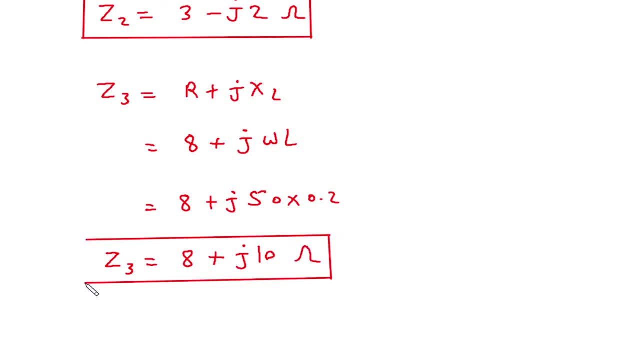 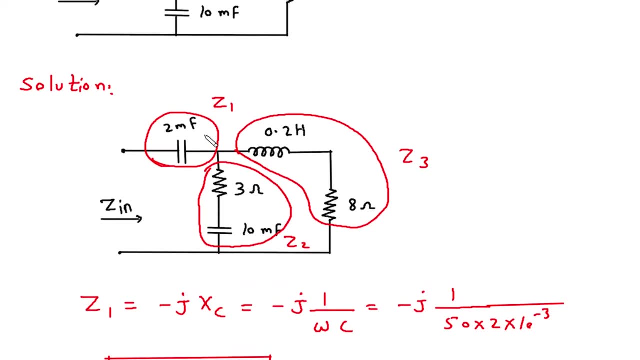 Unit is ohm. Now we have the value of Z1, Z2.. Now we have the value of Z1, Z2.. Now we have the value of Z1, Z2. And Z3.. Now, here we can see this: Zin is equal to, Zin is equal to Z1, Z1, plus now this Z2 and 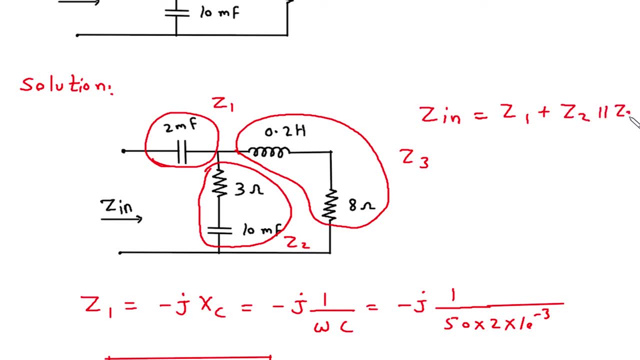 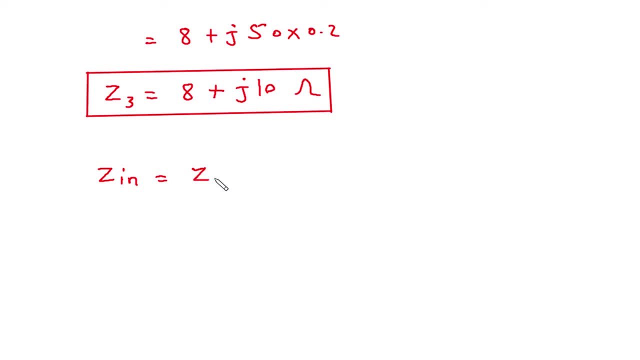 Z3 are in parallel, So Z2 parallel with Z3. So from this we can say: Zin is equal to Z1 plus Z2 into Z3, because Z2 and Z3 are in parallel and Z3 is equal to Z1 plus Z3.. 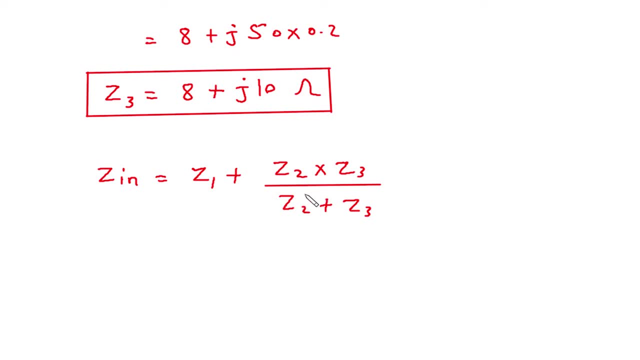 So this is our starting value. Now, this is our starting value, So we can understand it comes as we have taken both з1 and z2, this one comes as the same value. z gave 3 times the value 2 and z1 only gave y1 to z3 plus z3 is now a minus 10th of that. 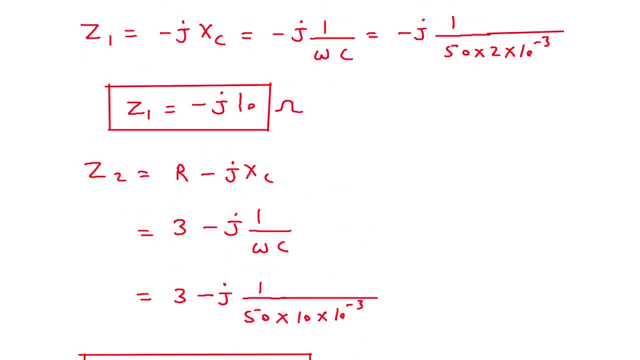 value z1 is x? z5.. z1 is xz5.. zx, that will be 0.. Here, the every place of any limb is close place of any limb, at any place of any limb: 1.. here, both, this is 0.. 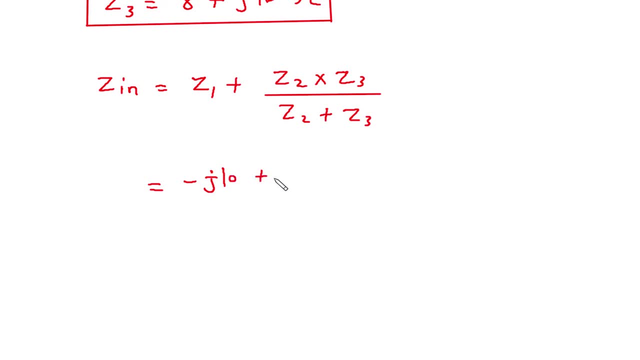 now xz5 happens to be. So z1 is equal to obrigado, Skin is equal to 0.. z2 is equal to 0, 3 minus j2, 3 minus j2 into z3, z3 is 8 plus j10 divided by same 3 plus 3 minus j2. then 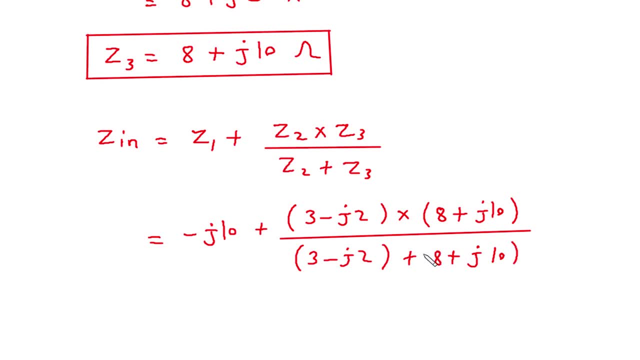 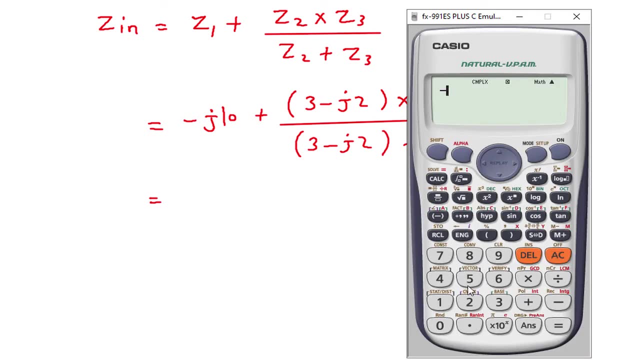 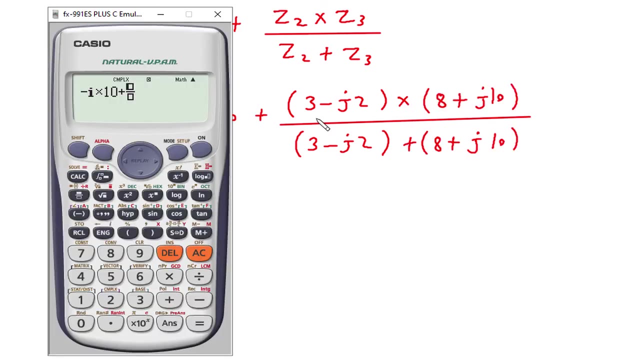 plus 8 plus j10, now we will directly solve this using calculator. so this will be minus i into 10, then plus now in bracket, 3 minus 2 into i, 3 minus 2 into i, then into 8 plus. 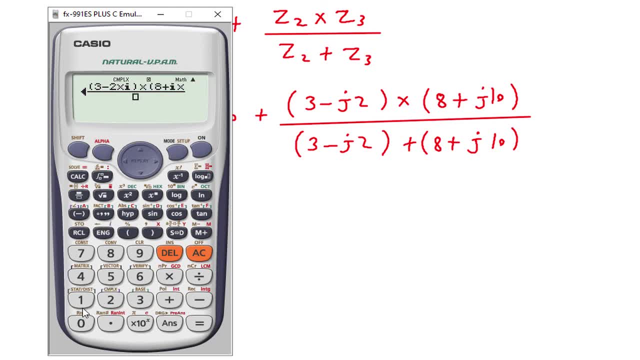 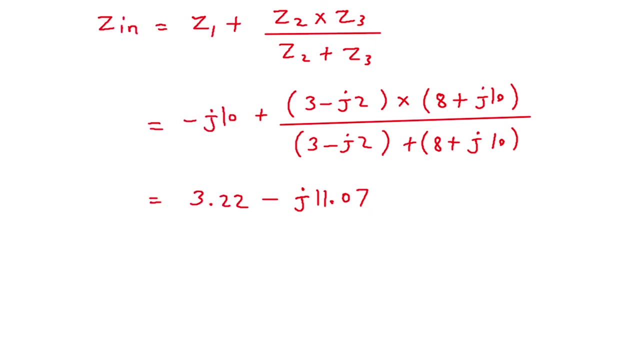 i into 10, divided by 3 minus 3 minus i into 2 bracket, then plus 8 bracket, bracket 8 plus i into 10.. So it is 3.22, 3.22, then minus j, 11.07. this is the value for Zin, the unit. again, here is: 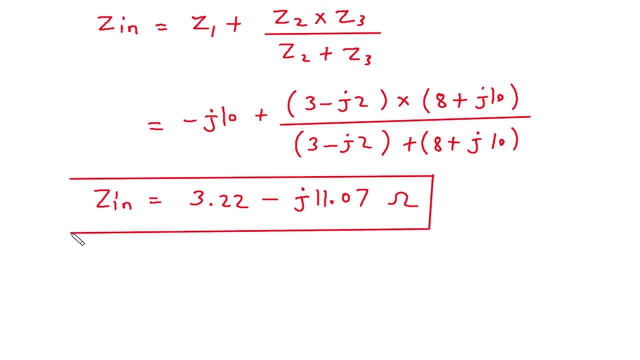 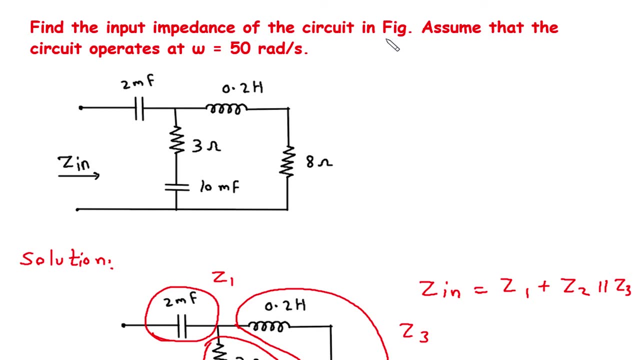 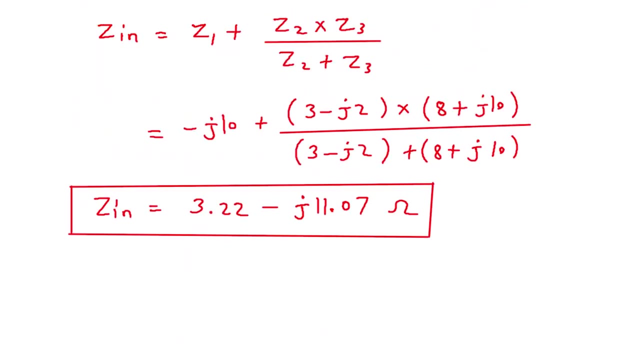 Ohm. so what we have to find, we have to find: find the input impedance of the circuit in figure. assume that the circuit operates at Omega is equal to 50 radian per second. so this is the final value of Zin.